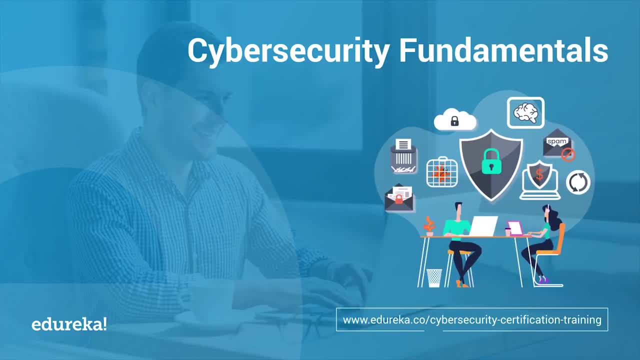 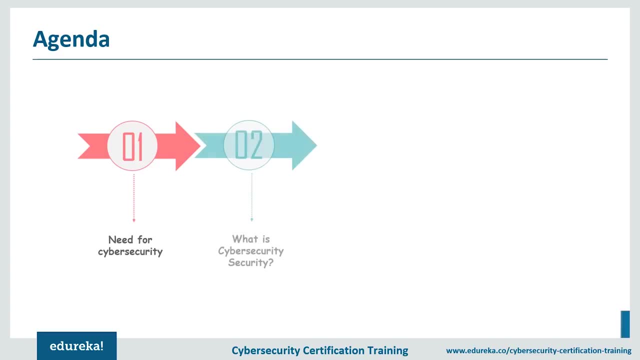 any delay. let's go ahead and take a look at topics that we will be talking about in this session. So, guys, we will begin by having a brief discussion on what is the need for cyber security. Then we will take a look at what cyber security actually is and then discuss its fundamental. 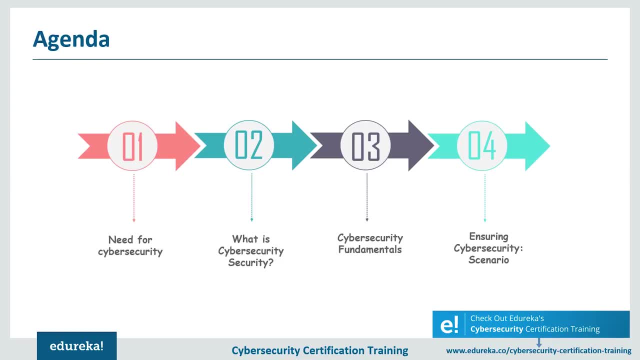 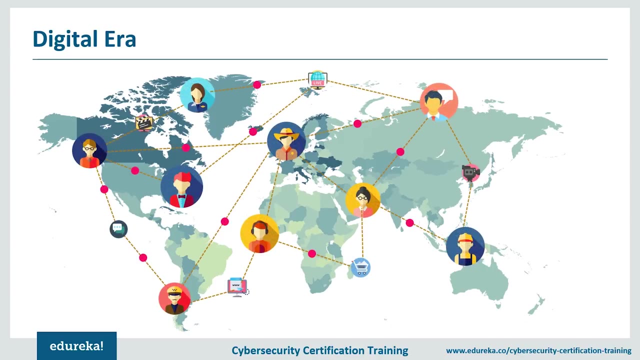 concepts. And finally, we will see how cyber security is ensured with the help of real world scenario. So I hope agenda was clear to you guys. Let's get started then. Internet today informs, entertains and connects us. It's the backbone of global economy. Our devices, which 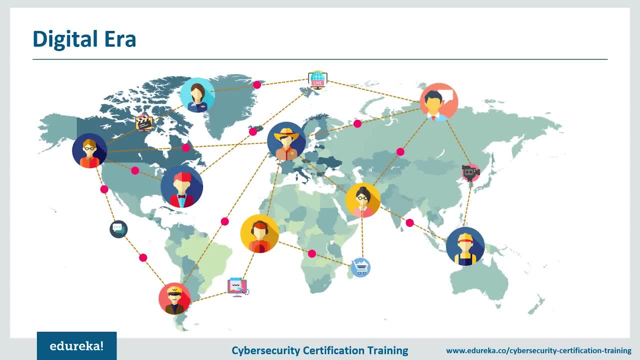 are connected through this internet and other networks open up a world of possibilities in front of us. For example, we can access information we need without having to keep it on our devices permanent. We can easily communicate with others who are on the other side of the world without 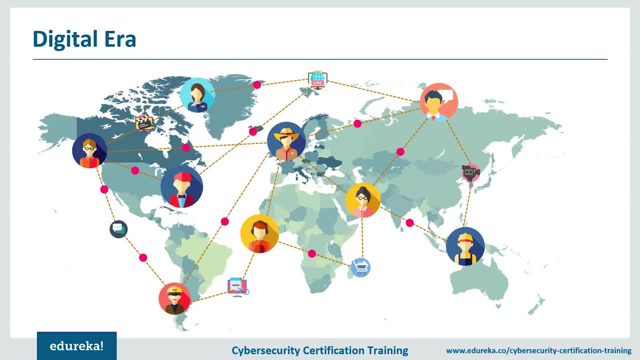 any glitches. These connected devices form the network that help us to run our lives, But these connections also leave our devices vulnerable to damage and our information vulnerable to theft. For example, cyber criminals are in business of stealing sensitive data like contact numbers, credit card information, bank account details that they sell to third parties for profit. 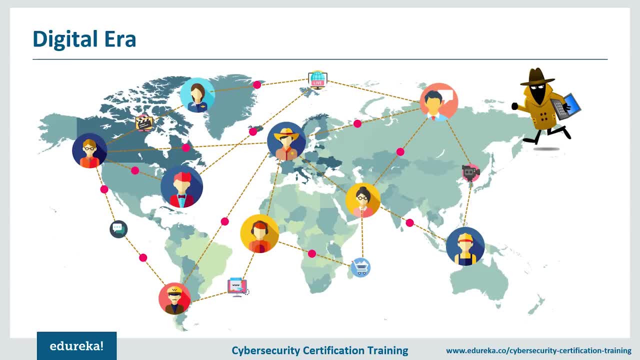 And then there are malicious hackers with personal enmity hack into systems to expose the host vulnerability. The hacktivist, inspired by their political and social activism, hacks systems opposed to their ideology and mindset. So, guys making use of these vulnerabilities that are present in internet's. 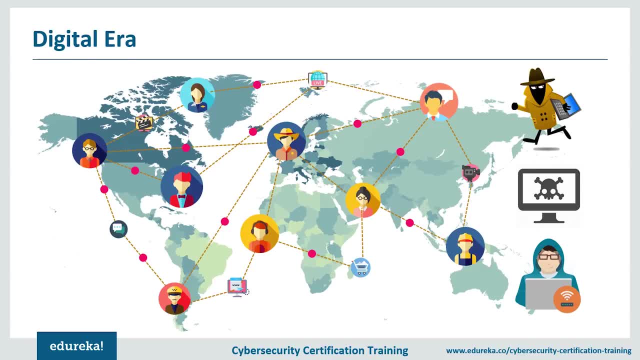 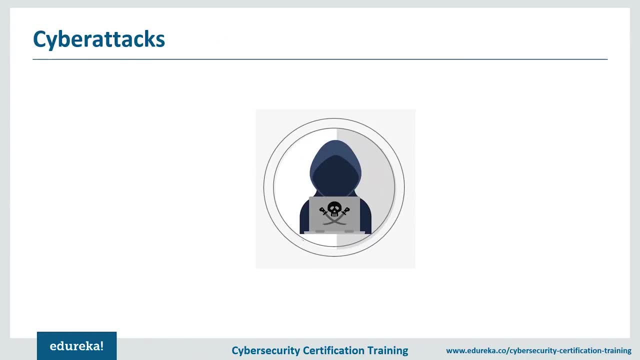 architecture. people are trying to initiate attack in the cyberspace. We call them cyber attacks. Now let's take a look at few popular cyber attacks that have terrorized the world till now. To begin with, there is malware. Well, if you have ever seen an antivirus alert pop up on your screen, 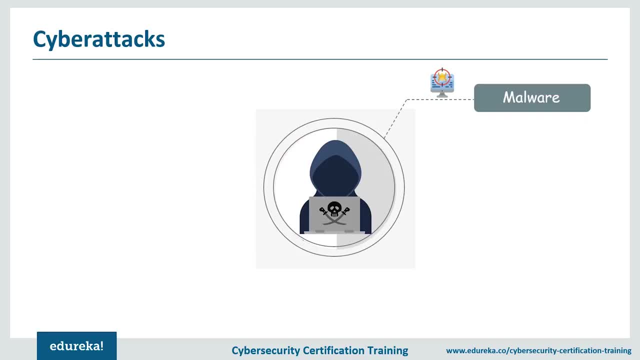 or, if you have mistakenly clicked on it, you can see that it is a cyber attack On malicious email attachment. then you have had a close call with malware. Malware, basically, is a term which is used to describe malicious software, including spyware, viruses, worms, different. 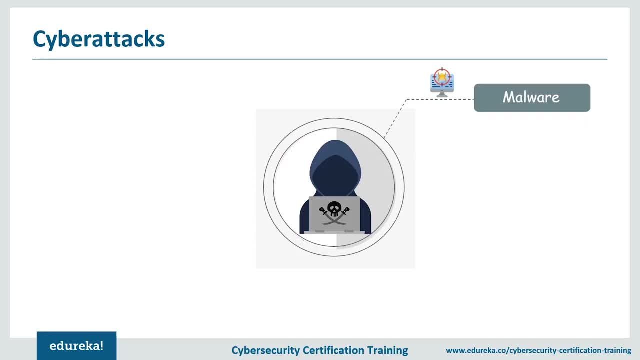 kind of trojans that are injected into your computer to corrupt it. And then there is something called phishing. In a phishing attack, an attacker may send you an email that appears to be from someone you trust, like it could be your boss or a company that you do business with. In this email, 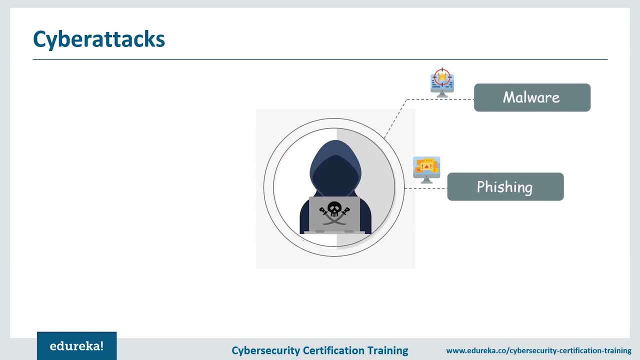 you will find an attachment to open. There is a link asking for you to click on, And as soon as you do that, you're giving leeway for attacker to exploit your computer. And then there is man in the middle attack. It is also known as eavesdropping. 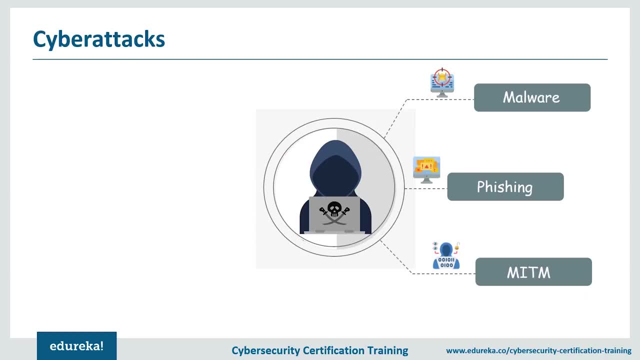 attack. Here attacker inserts himself as a third party into a two-party transaction. Once the attacker interrupts the traffic, he can easily filter, manipulate and steal your data without you knowing anything about it. Moving on, we have denial of service attack. Here attacker floods. 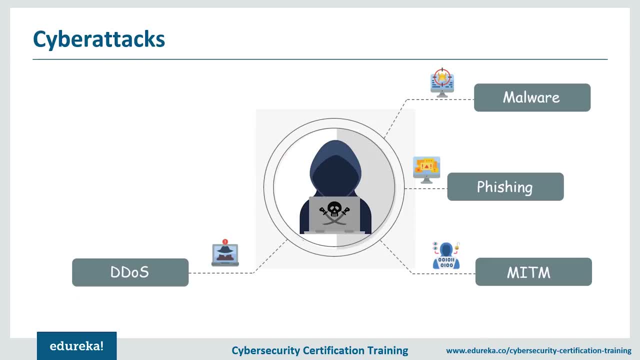 a website with more traffic than it can handle. This will make it impossible for the website to respond to legitimate visitors who are trying to access it. And then there is malvertising. It is the use of online advertising to spread malware. It typically involves injecting malicious advertisements into legitimate online advertising. 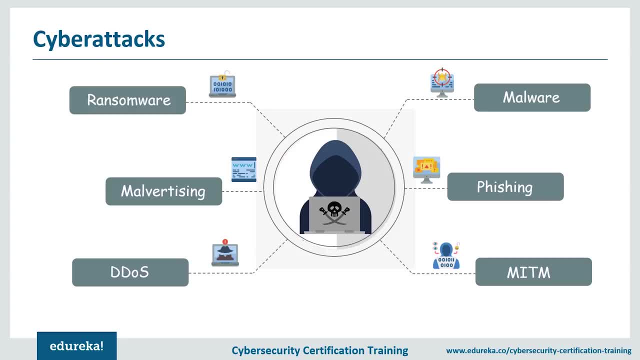 networks and web pages. And finally, there is ransomware. Ransomware, basically, is a type of malware that prevents users from accessing their system or personal files. If the user want to regain access, then you'll have to pay the price. If the user wants to regain access, then you'll have to pay the price. 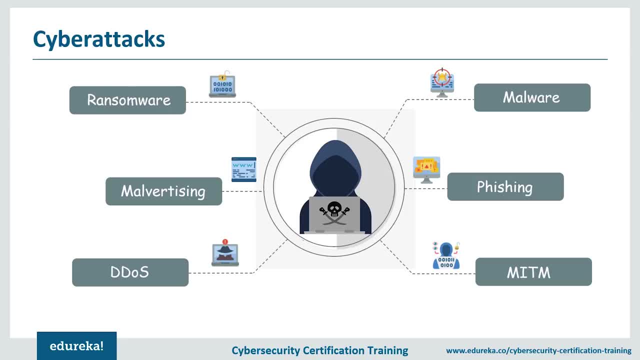 The ransom that the attacker is demanding. And today, most of the time, ransomware criminals order that payment be sent via cryptocurrency or credit card. So, guys, these are just few major type of cyber attacks that are there. There are others out there that are traumatizing the 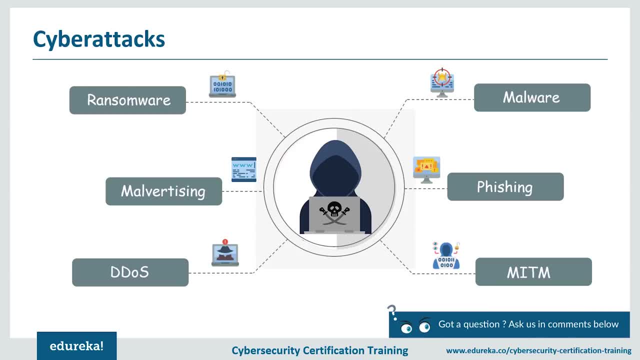 cyberspace. Cybercrime is a global problem that's been dominating the news cycle. It poses a threat to individual security and even bigger threat to large international companies, organizations, banks and government. But the good thing is that, even with this flawed internet, there are simple things that we can do. 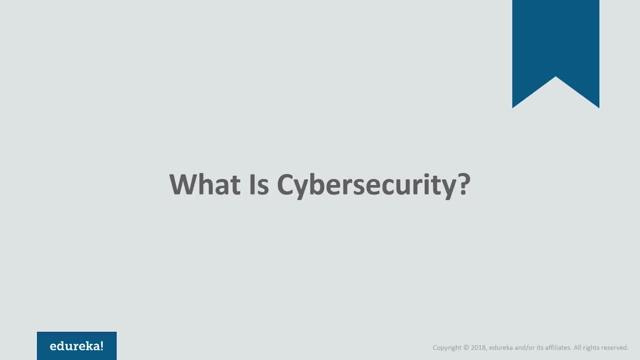 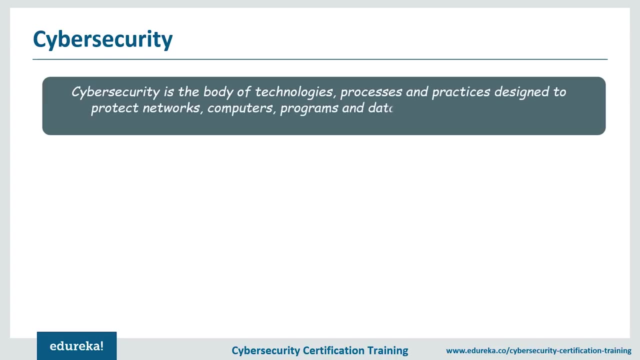 to protect ourselves from these attacks. This is where cyber security comes into picture. In simple terms, cyber security is defined as techniques and practices designed to protect your data, And when I say data, I mean digital data that is stored, transmitted and used on an 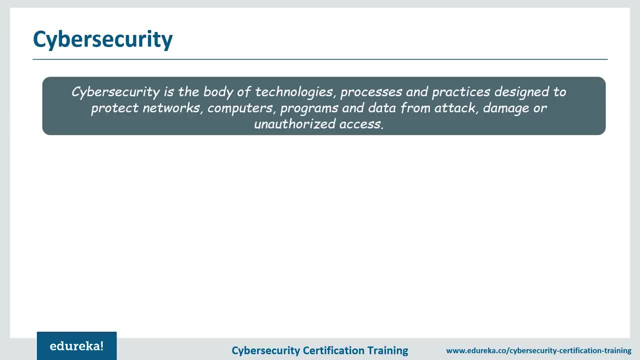 information system. After all, this is what criminal wants, right? The data, The network servers, computers and other online gadgets are just mechanisms to get this data. Ensuring cyber security requires the coordination of efforts throughout an information system, And this includes application security. It mainly 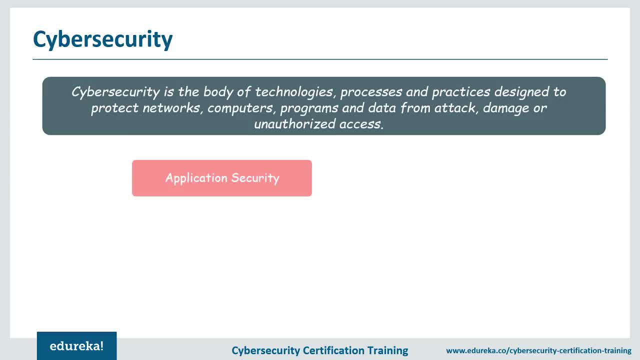 focuses on keeping software and devices free from cyber threats. And then there is information security. It is basically protecting the integrity and privacy of data, So you're protecting organizations from possible data breaches here. And then there is network security. It is practice of 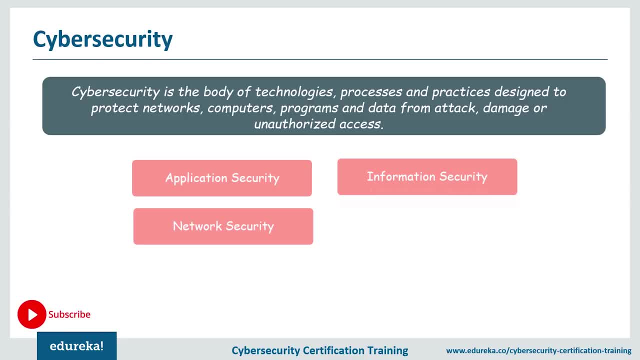 securing a computer network from intruders, whether it could be targeted attackers or simple malware Moving on. there is operational security. It includes all the processes for handling and protecting data assets, The permissions which users usually have when they're accessing a network, and the procedures that determine how and where data must be stored and shared. 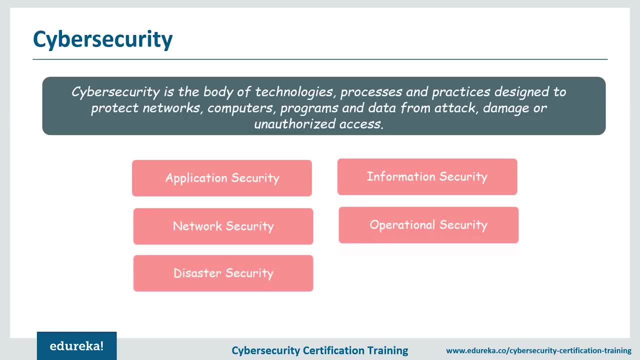 all fall under this category. And then there is disaster recovery and business continuity. they define how an organization responds to a cyber security incident or any other event that causes the loss of operation and data. and finally, the most important thing, end-user education. it addresses the most unpredictable cyber security. 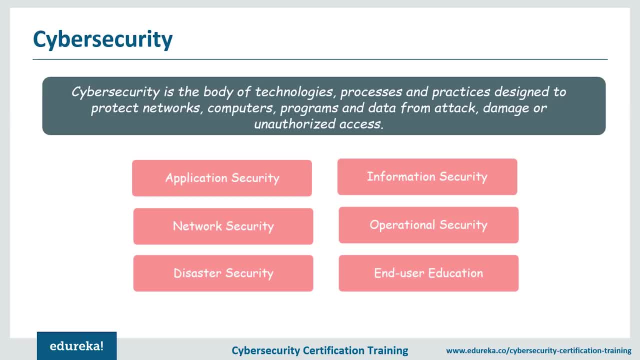 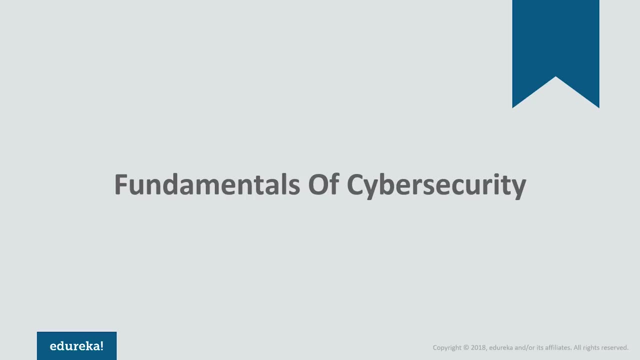 factor, which is people teaching users to delete suspicious email attachment, not plug in unidentified USB drivers and various other important lessons, is very vital for the security of any organization that there is. so, guys, earlier I said that cyber security is set of techniques and practices employed to protect data. 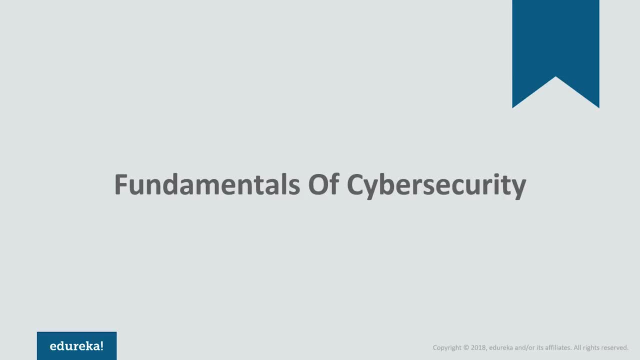 But what are we actually protecting data here from? we are protecting data from unauthorized access, unauthorized modification and unauthorized deletion. These three terms are similar to what we know as CIA triad and cyber security. CIA basically stands for confidentiality, integrity and availability. Now let's explore the CIA triad. 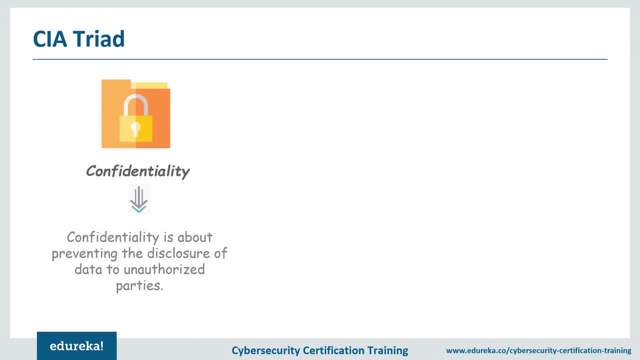 So confidentiality is exactly What It sounds like. keeping your information secret. It is the protection of information from unauthorized people and processes. Let's consider a simple example. Would you like the thought of your private health information or financial information falling into some stranger's hands? 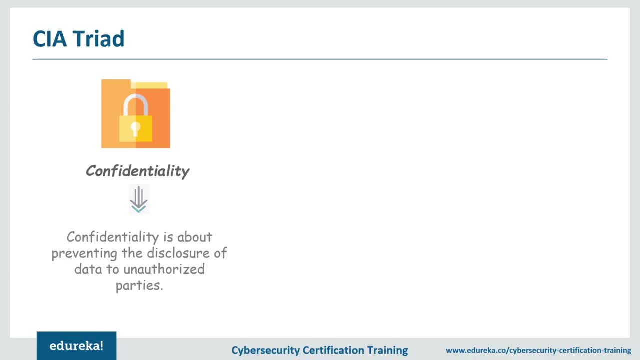 Whoa, definitely not right. Similarly, no business owner likes the thought of a business information being disclosed to competitors. information is a valuable asset. integrity is when the information that is stored in a system Is very accurate and highly reliable. integrity is protection of information from intentional or accidental, unauthorized 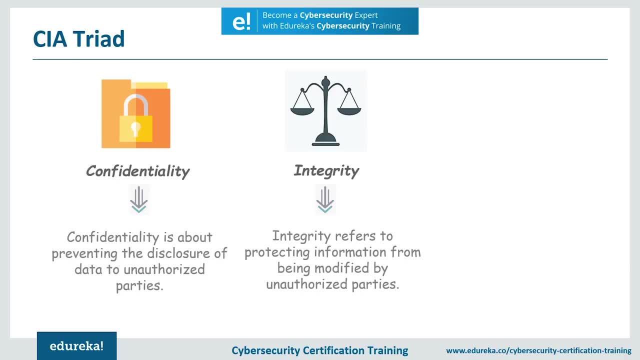 modification. For example, if a hacker were to break into a banking website and change its balance from $1 to 1 million dollar, Integrity of site is now lost. The final component of CIA triad is availability. Availability is assurance that systems and data are accessible. 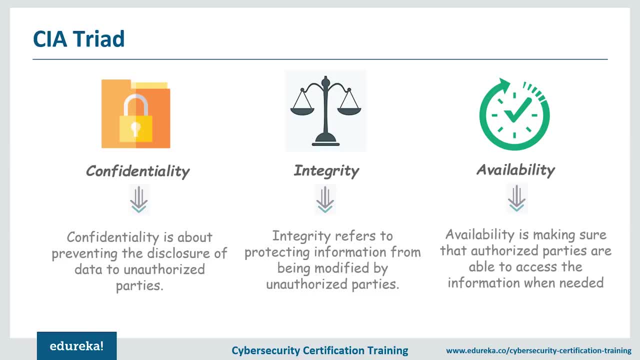 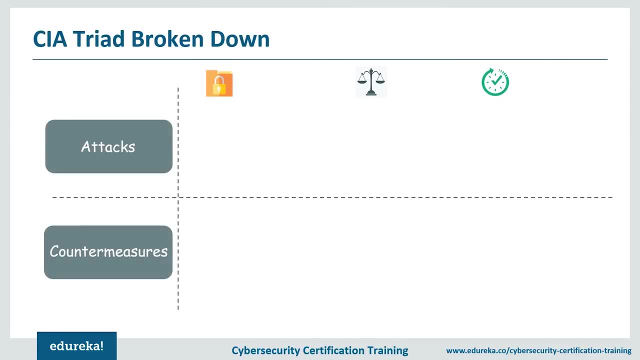 by authorized users whenever they need it. So if it cannot Access the data whenever we need it, We are definitely not secure. So, guys, now you know what CIA tried basically means. now Let's take a look at what kind of attacks can be made on the 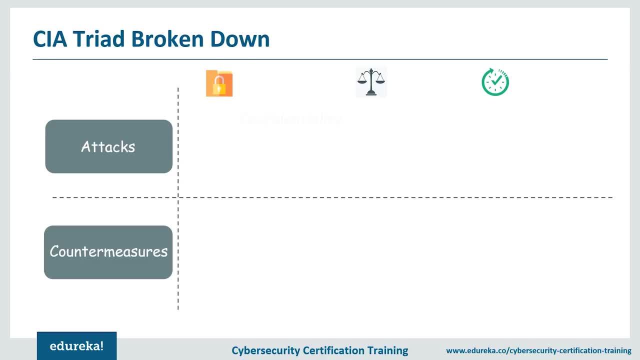 CIA tried in real world on how we can live in there. Let's begin with confidentiality. attacks and confidentiality include cracking poorly encrypted data and employee knowingly or unknowingly putting sensitive data on removable media such as SD cards when drives and giving it to unauthorized parties. and then there is doxing, which is basically leaking private. 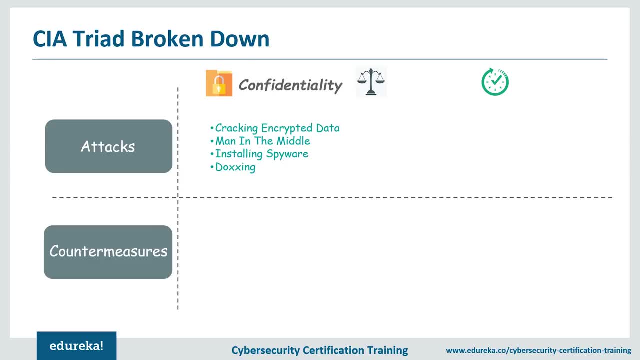 information about an individual or an organization in order to do harm. Now, the best way to keep your information secret is to make sure that there is strict access control, that is, only people who are allowed to access data can access it. and another way is to encrypt any data that's being transmitted from one 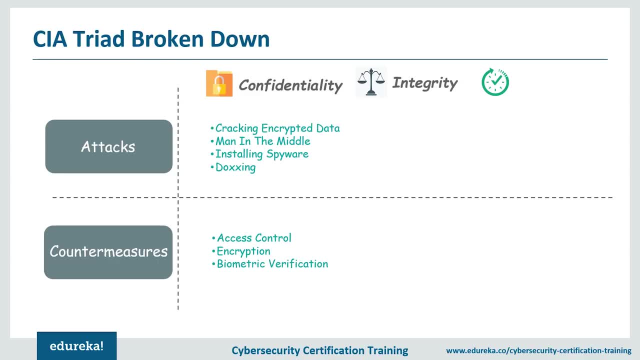 position or one place to another. Now, Integrity. attacks on Integrity include penetrating a web server in order to embed malware into web pages to corrupt the system, or maliciously accessing the financial server in order to falsify financial records. or hacker turning your machine into a zombie computer so that he can control your. 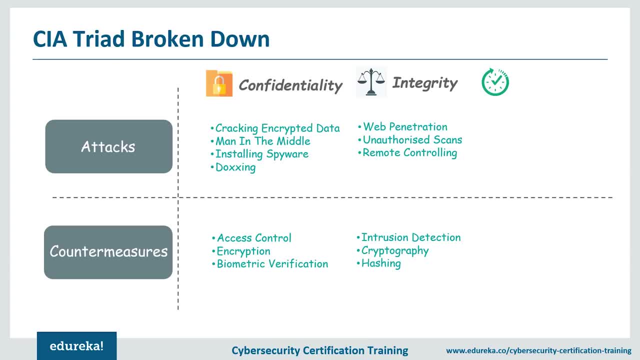 computer without you knowing about it, and the best way to upload the Integrity is to use cryptography and then ensure intrusion detection. Well, if you're wondering what intrusion detection it, it's the act of detecting when hackers can carry out actions that might compromise the Integrity of the system and finally threats you. 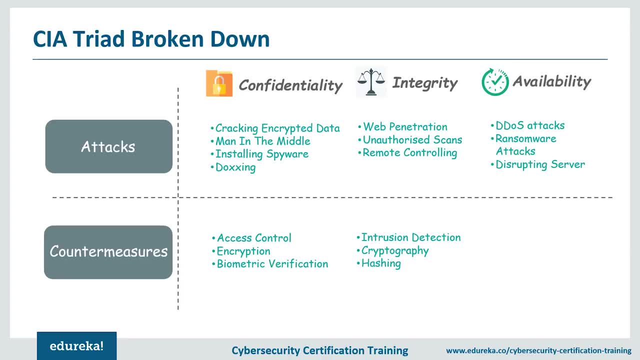 should be aware of when thinking about availability: is denial of service attack or distributed denial of service attack? We already talked about it earlier. Basically, denial of service attack is one where enemy will flood your computer and internet connection with traffic so that the legitimate users can't access any information that. 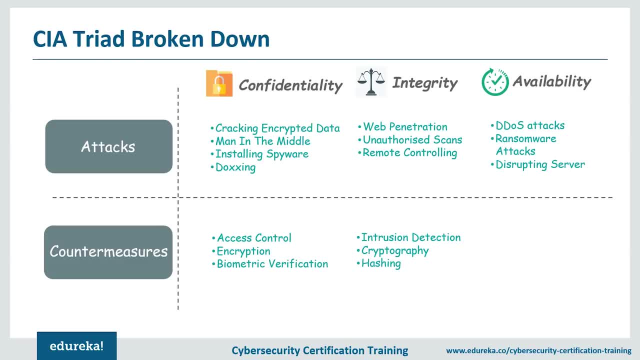 there is on website, and there are other attacks as well, For example, ransomware attack, which encrypt data on targeted computers so that the authorized parties cannot use it, and then deliberately disrupting a service Server rooms power supply so that the servers go offline. now a few ways you could protect yourself from these attacks are: 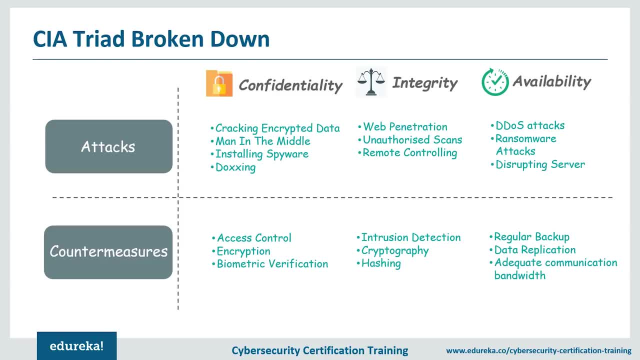 by using antivirus software, or you could install spyware detection and spyware remover softwares as well and you could start using a firewall. So, guys, the CIA triad is very fundamental concept, and security, confidentiality, Integrity and availability all have to work together to keep your information secure. but don't 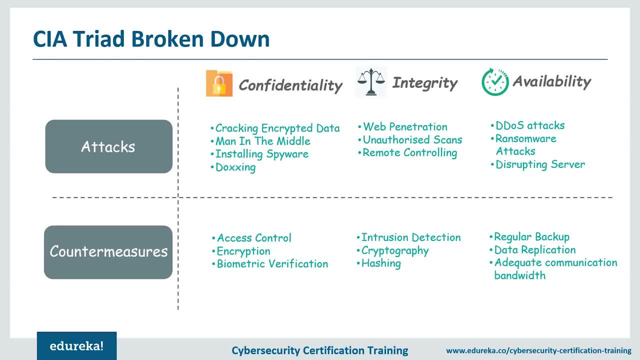 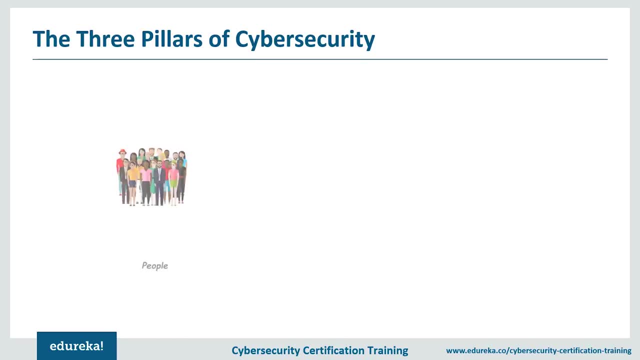 think for one minute that these are the only factors to be considered while talking about security. Now let's talk about other three pillars of security. to begin with, the most important concept: people and individual. It could be me, or it could be you- play a very important role. 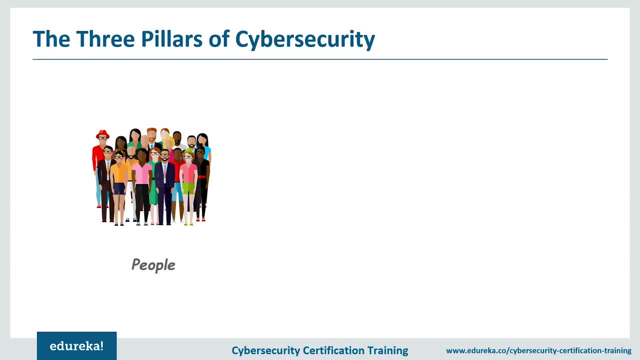 when it comes to security. Every employee needs to be aware of their role and preventing and reducing this ever-ending cyber attacks. The specialized technical cyber security staff need to stay fully update with later skills and qualifications to mitigate and response to cyber attack easily. So, guys, people play a very important role when it comes to. 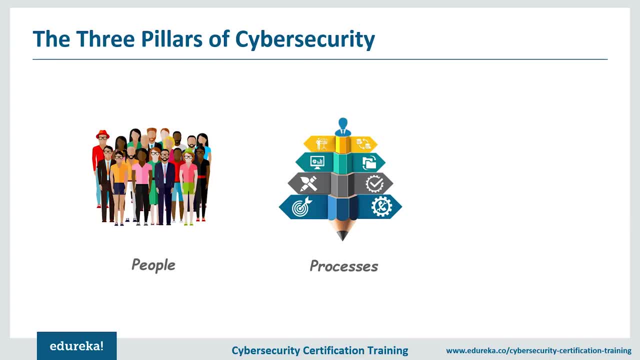 security. moving on, We have processes. processes are crucial and defining how the organization's activities, roles and documentation can be used to mitigate the risk of organizations, information and data. cyber threats keep changing quickly, So processes need to be continually reviewed and updated to be able to adapt to with them. 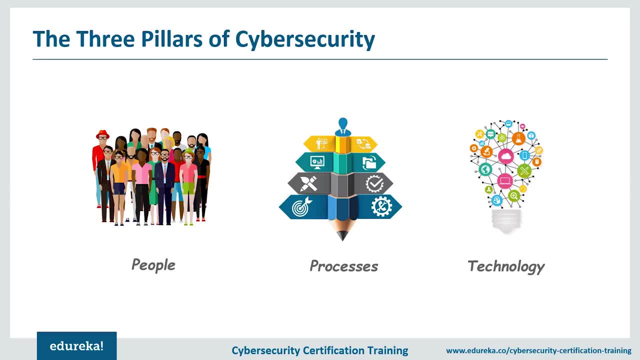 And finally, technology. technology plays a very important role. technology can be deployed To prevent or reduce the impact of cyber risk, depending on your risk assessment and what you deem an acceptable level of risk. So, guys, now that we are aware of what cyber security is and 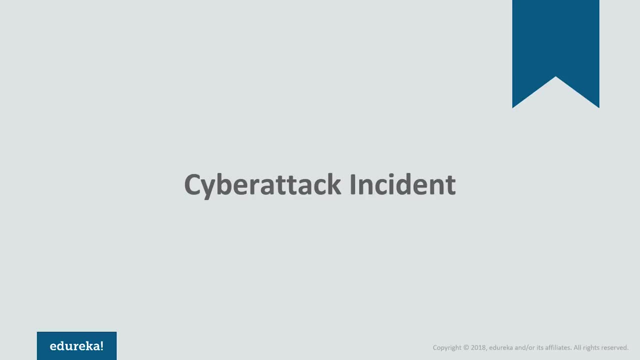 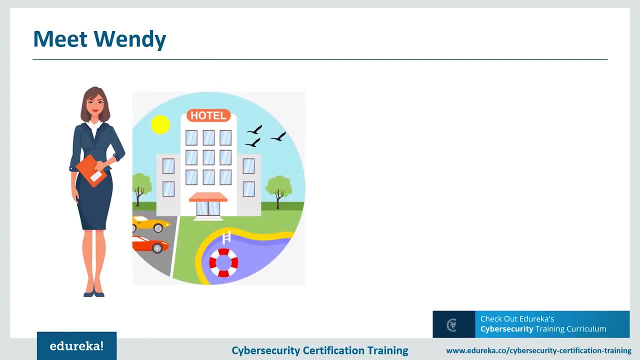 its fundamentals. Let's take a look at real-world scenario to understand how cyber security is injured. Meet Wendy. She owns a successful hotel and spa because everyone needs an escape from the stressful life once in a while. right Now, being the owner of successful spa means that her 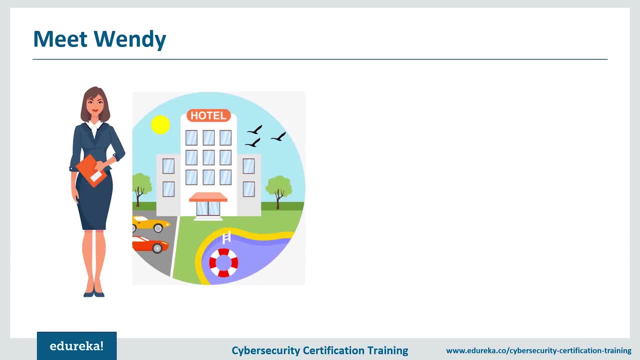 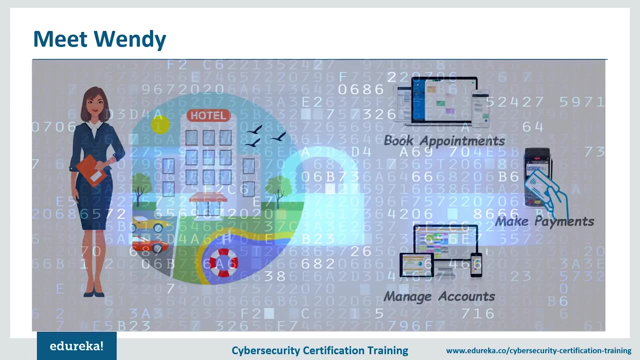 clients are trusting her With their personal information, and she uses different kind of technical systems to book appointments, make payments and keep track of her financial accounts. on top of that, to keep it all safe, She has an elaborate IT security system protecting everything, But unfortunately it's not secure enough. 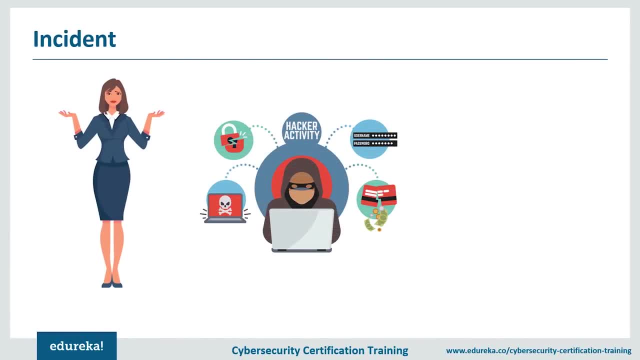 Wendy's business is targeted by hackers who are determined to break and hold the business information hostage. because of this, Wendy's business has come to a halt. She can't make appointments, Can't process payments and a client's person information is exposed. and on top of that, hackers are asking her for a. 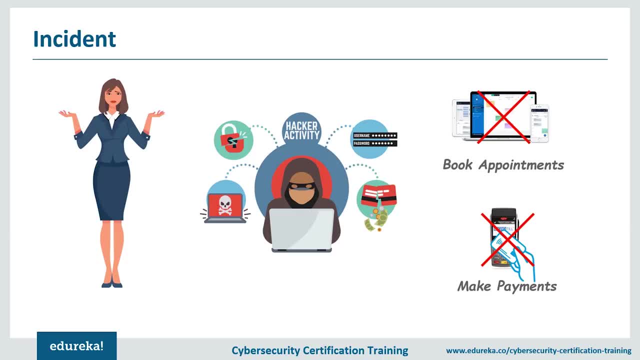 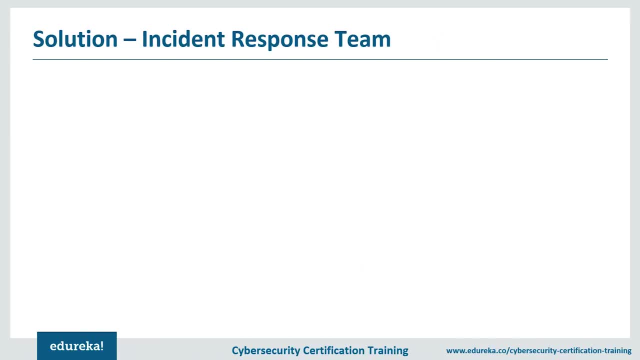 heavy ransom. So what would you do if you are in Wendy's place? Well, Wendy doesn't want to pay hackers, So she decides to hire instant response team from a very popular security company. This incident response team mission, basically, is to prevent serious loss of profits and your public confidence, and 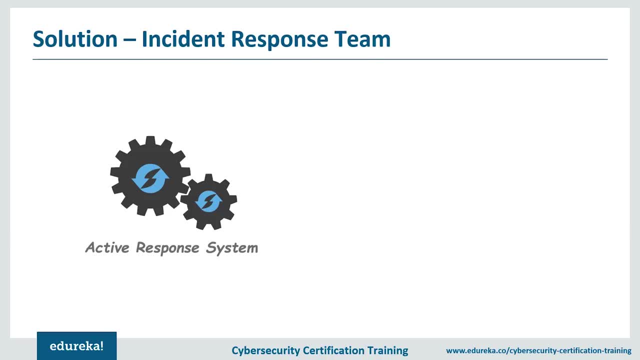 protect information assets for business like Wendy's. But how does this IRP team actually achieve it? So, as first step, IRP team will identify the source of security breach. then IRP team orchestrates China events that ultimately prevents from encountering a serious security disaster. 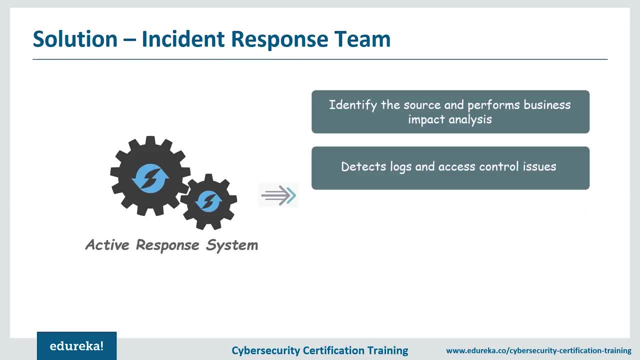 They detect logs and access control and contain the threat part so that Wendy's company can avoid further damage. after the attack is contained, the team identifies the data that has been stolen or compromised during the incident. after that, the team prioritizes recovery To project Wendy's business from further attacks. 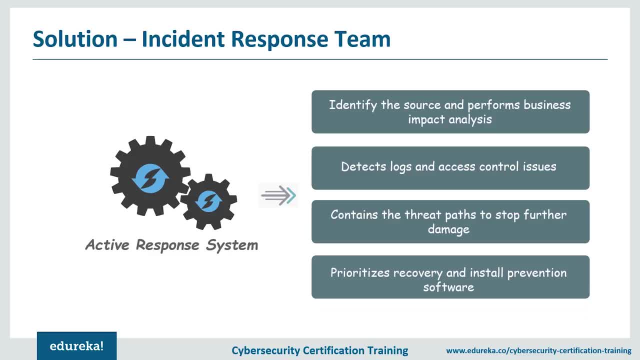 Now Wendy's customers can continue their spa day without any hassles. in the past, security beach of this nature would have required Wendy to contact several agencies and third parties to solve the problem. in the worst case, Wendy might have had to pay hackers the amount they demanded for, but IRP platform organized all of these people. 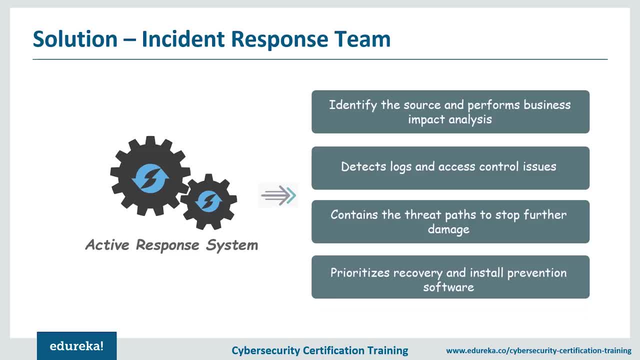 processes and technology to identify and contain the problem in very limited amount of time. So, guys, today, if you have reached the position in which cybercrime is so sophisticated, it seems almost impossible to prevent. the emphasis is now on how an organization response once it has been breached. 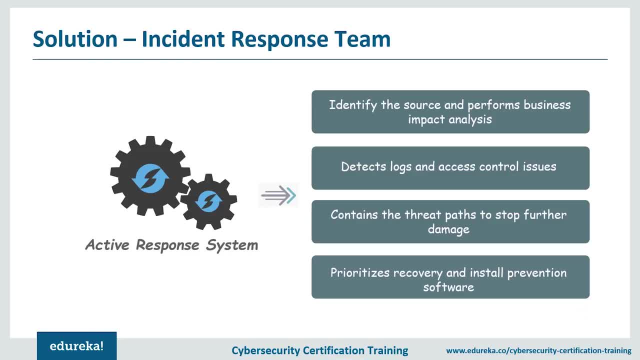 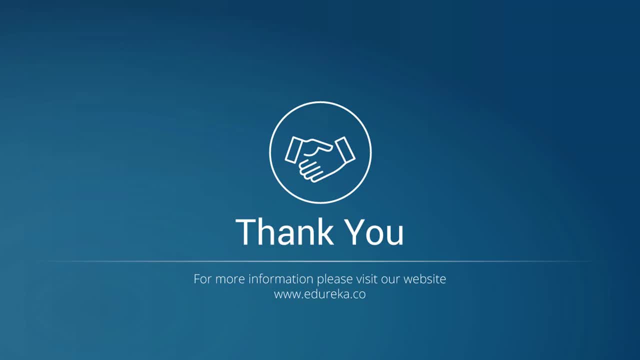 Well, we can't prevent every incident that there is. we can easily control how we manage the aftermath so that we're prepared and practiced in the process of response. So this is it, guys. We have reached the end of the session. I hope the session was informative and now you know.